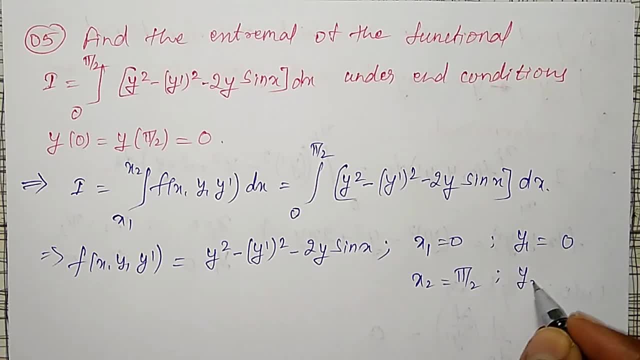 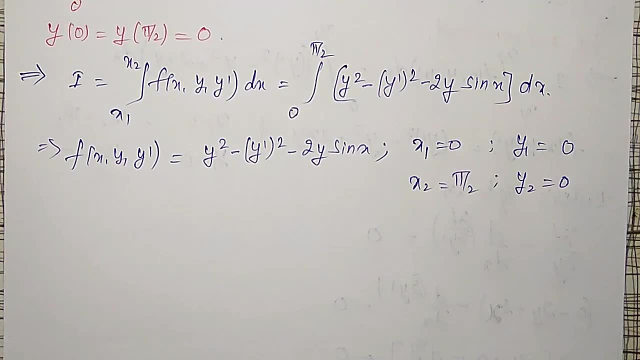 x2 is equal to pi by 2 and corresponding y2 also equal to 0. they have given Then from this one the condition to find out the extremal, the necessary condition. Euler's equation is given by necessary condition. Euler's equation is nothing but 0. 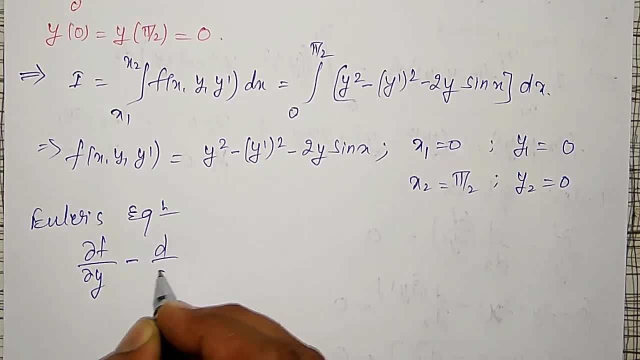 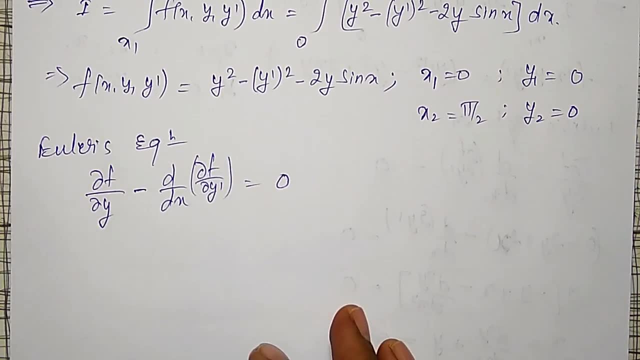 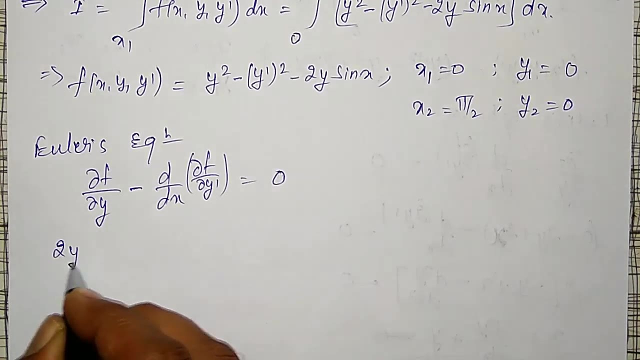 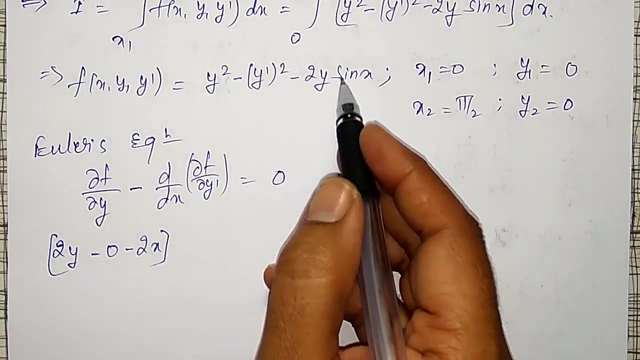 So 1 over dy by 2y minus dy by dx of dy by 2y, dash equal to 0.. What is my dy by dy From this one, differentiating this one partially with respect to y? Now, that is 2y minus 0 minus 2x is the partial derivative of f with respect to y minus dy. 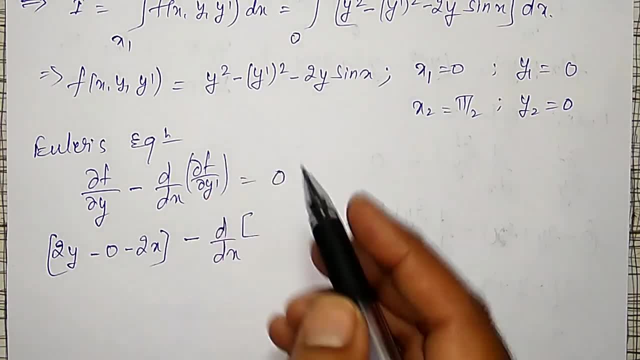 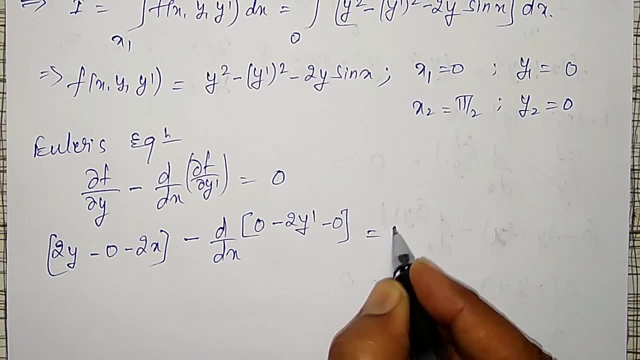 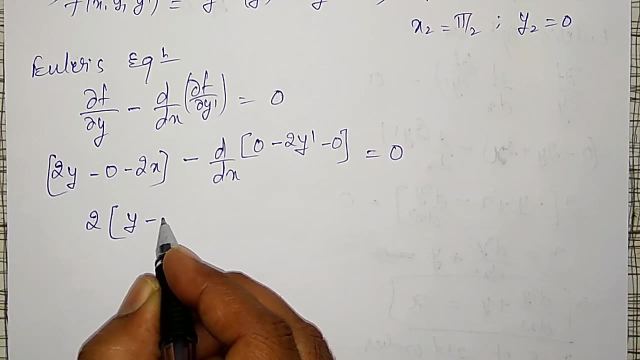 by dx partial derivative with respect to y dash. first one is 0 minus. this one is 2y dash minus 0, must be equal to. I can simplify and write this one as 2,. I can take common from both the terms y minus sin x. sorry, I have written here x. it should be sin x. y, sin x minus. 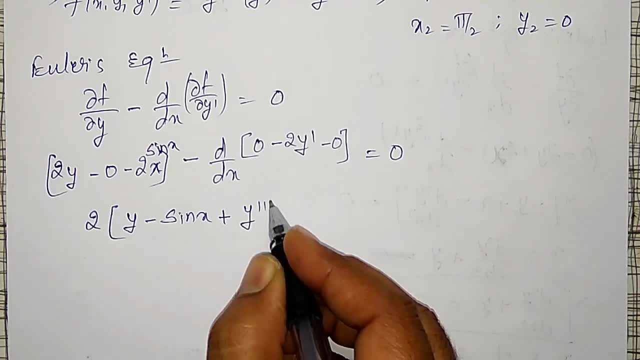 x of minus plus y double dash I can write. derivative of y dash will become y double dash. that implies what I can write. 2 will cancel other side. therefore y double dash plus y equal to sin x, I can write, which is the differential equation of a second order: 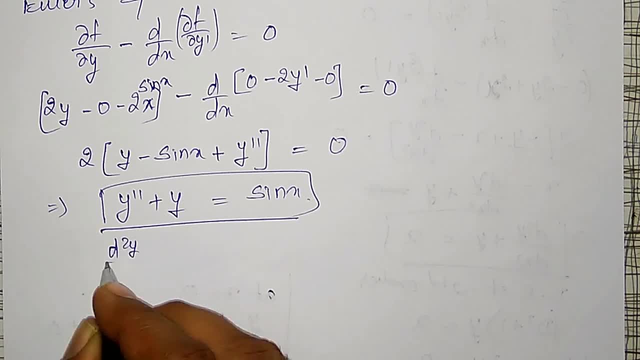 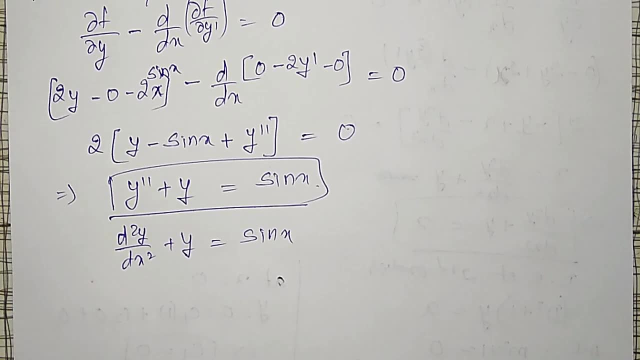 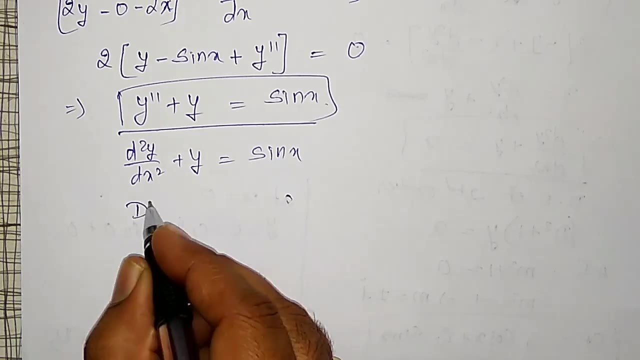 to solve this one. I can write this one as d square y by dx square plus y, equal to sin x. okay, now to solve the second order differential equation. I will substitute d square y, d by dx by d that over. I can write it as d square plus 1 into y, equal to sin x. therefore. 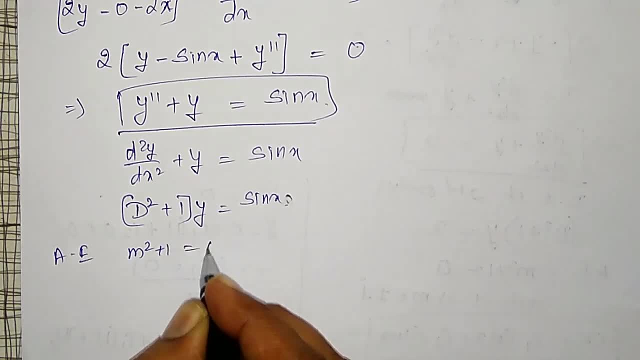 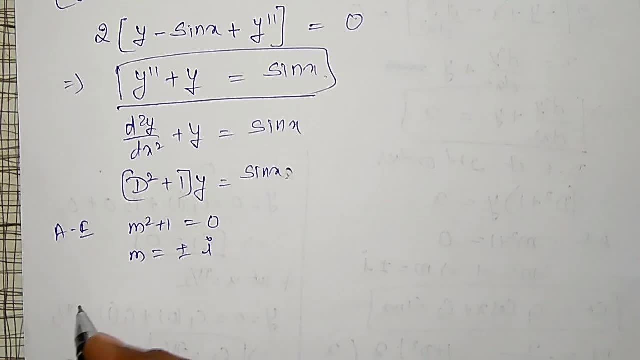 auxiliary equation is given by m square plus 1 equal to 0, therefore m is equal to plus or minus i. I can write: if m equal to plus or minus i is there, then cf is nothing but a sin x. okay, now to solve the second order differential equation. I will substitute: 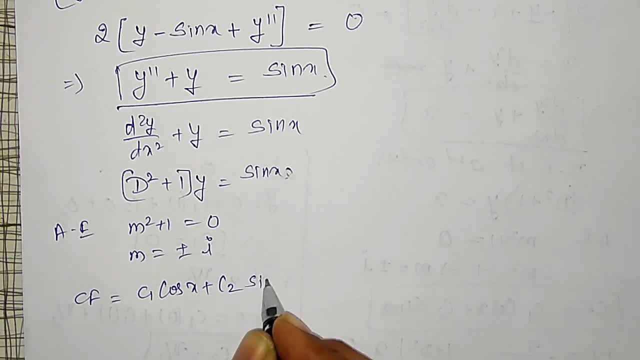 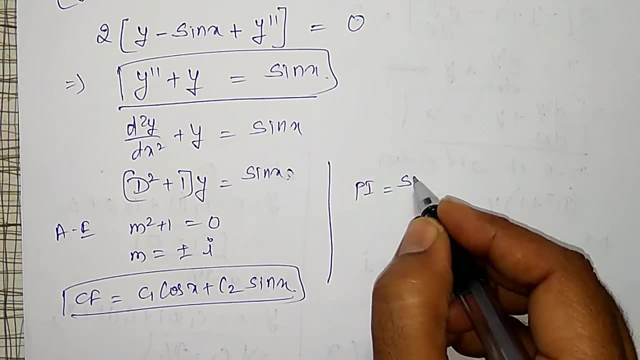 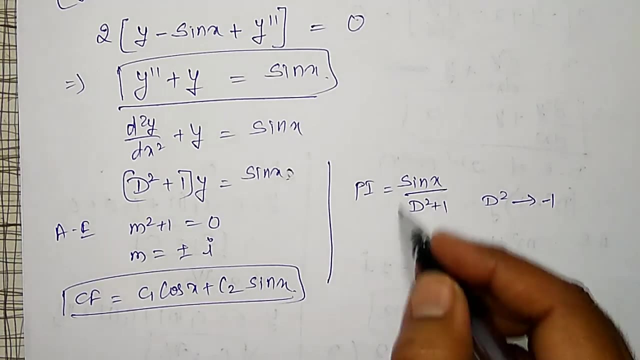 c1, cos x plus c2, sin x is my cf, then particular integral. I have to find out pi equal to sin x divided by d square plus 1, then d square is replaced by minus 1,. these are all things you have studied in second semester, or you can go through with my videos of second semester. 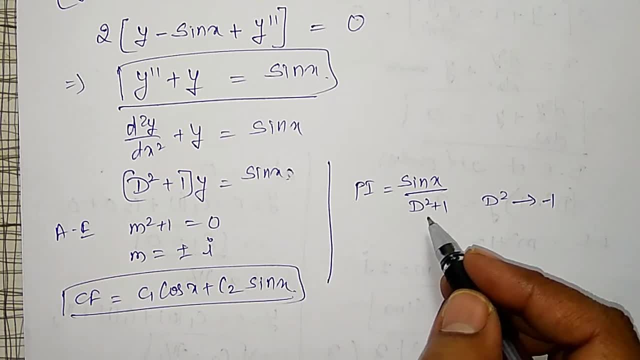 differential equations of higher order. there you will get how to find all these things now. which is equal to sin x by dx square plus y, by dx square plus y? equal to sin x divided by minus 1 plus 1,, therefore. which is equal to sin x divided by 0,, therefore, which? 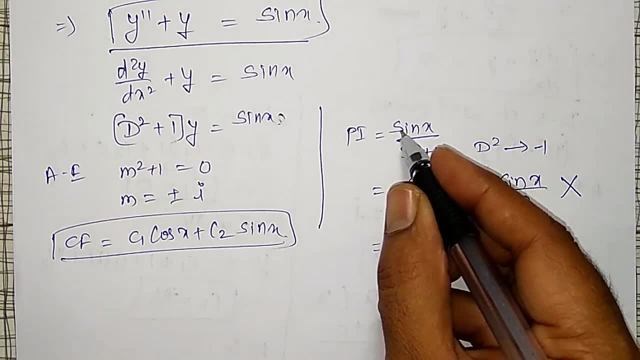 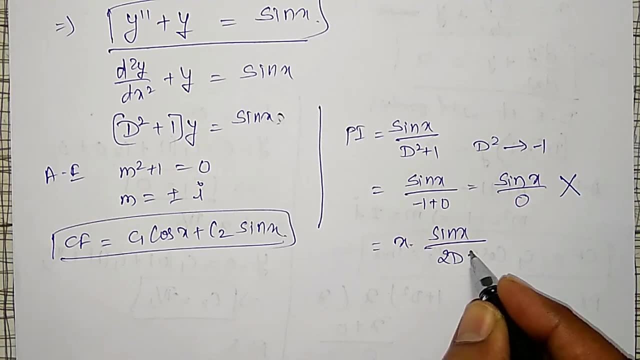 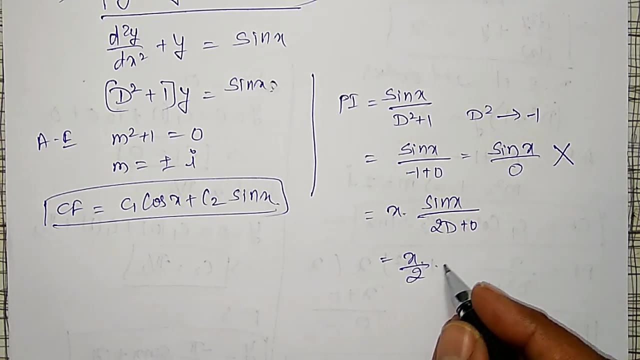 is not a particular solution, integral. therefore, what I have to do: multiply by x, sin x divided by, differentiate the denominator, that is 2d plus 0, okay, then this is nothing but x into x divided by 2, 1 by d is nothing but integration of sin x. okay, so this is nothing. 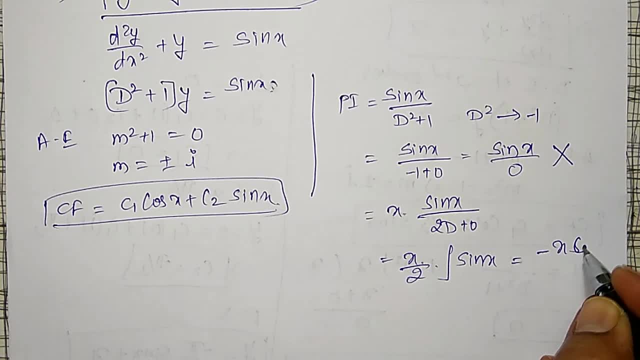 but x into x divided by 2, 1 by d is nothing but integration of sin x. okay, so this is nothing but integration of sin x. okay, so this is nothing but integration of sin x, which is equal to minus x into cos x divided by 2, integration of sin x is cos x minus. 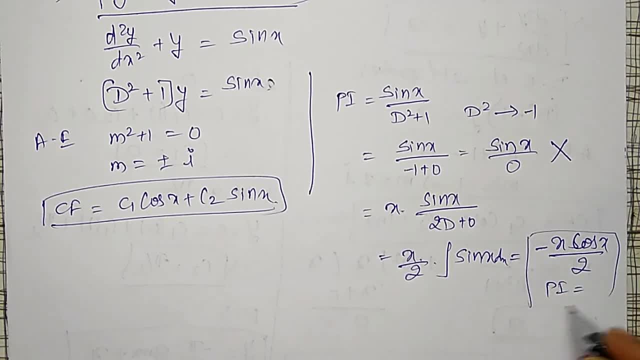 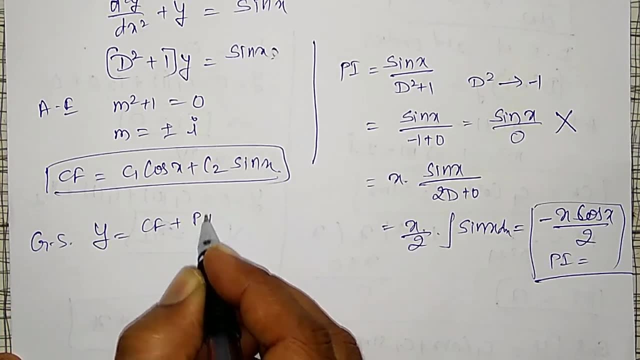 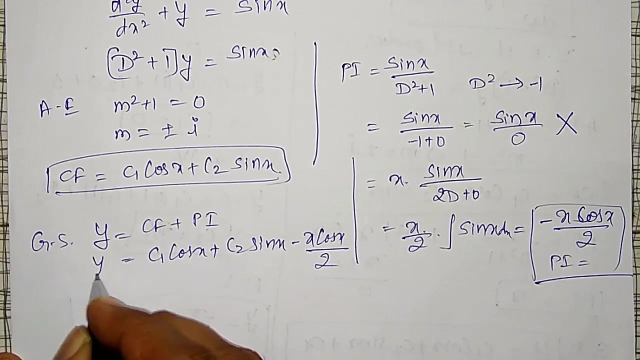 x. this is my particular integral. okay, therefore, general solution: y is equal to cf plus pi, that is cf. cf is c1 cos x plus c2, sin x minus x cos x. okay, so this is nothing but cf cos x divided by 2, is my general solution. okay, and using the initial conditions, I 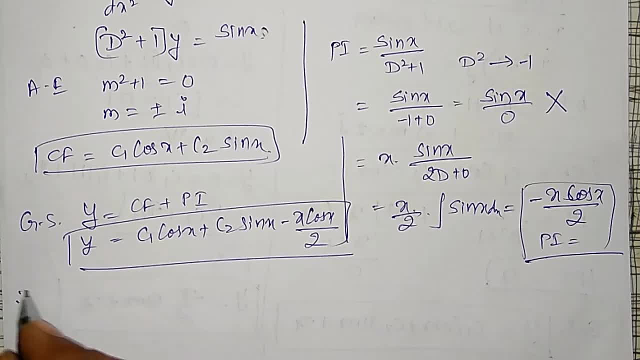 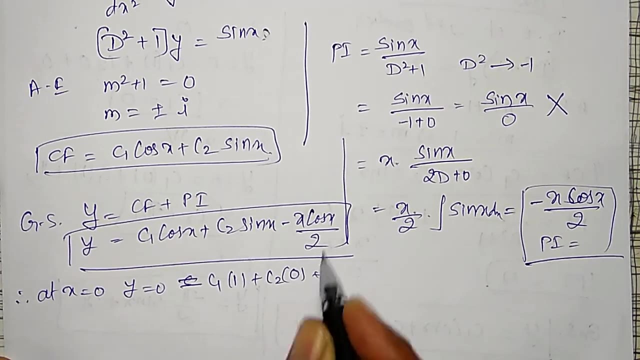 have to find the value of c1 and c2,, therefore at x equal to 0, y also equal to 0, substitute in this: x equal to 0,, which is equal to c1 into cos, 0 is 1, plus c2 into sin, 0 is 0 and. 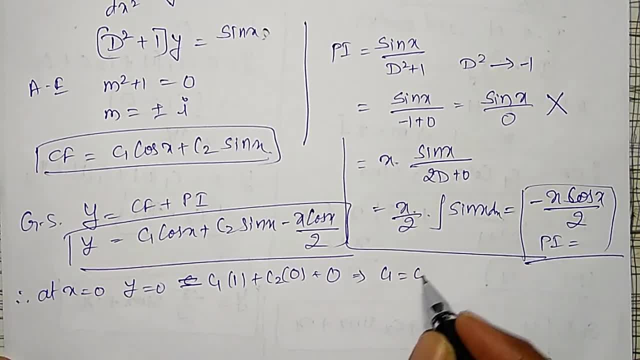 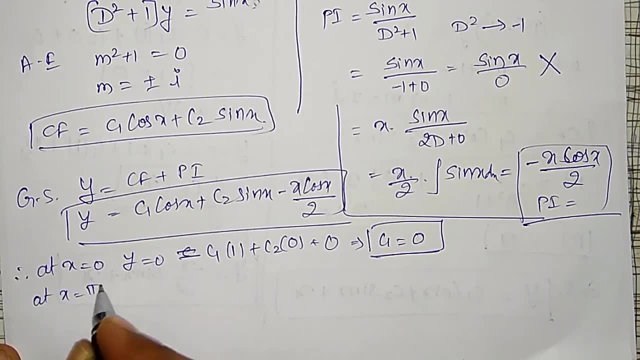 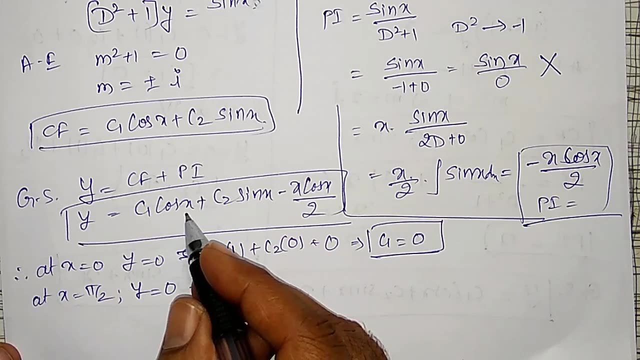 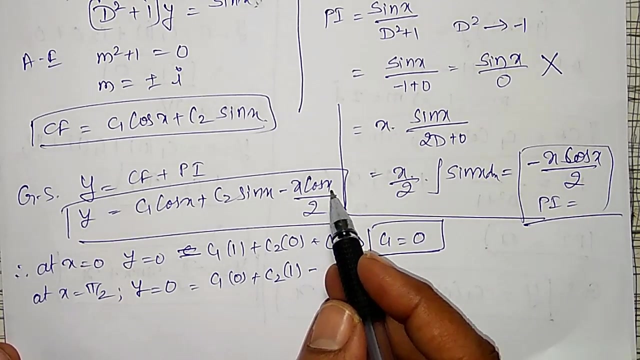 0,. therefore c1 is equal to 0.. 0 here c1 equal to 0,. next at x equal to pi by 2, y equal to also 0,. therefore c1 into cos, pi by 2 is 0 plus c2 into sin is 1 minus again cos pi by 2 is again 0,. therefore,